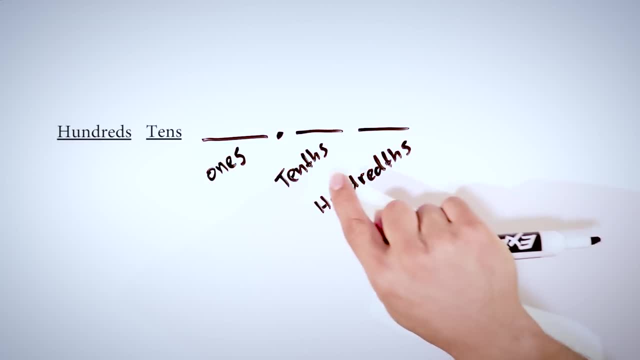 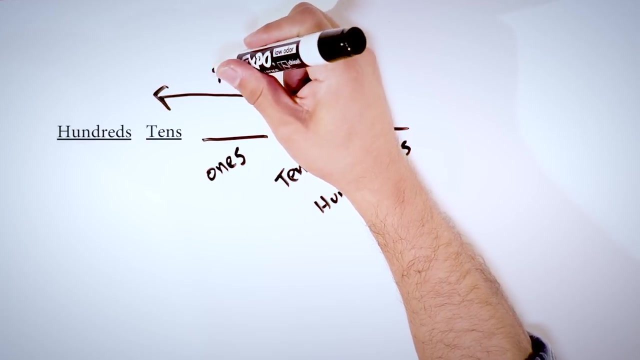 but they're different because these are tens and hundreds and, if you notice, the endings are different. So, like I said, these places are going to be less than the ones place because, as we know, when we go left on our place value chart, our values increase and as we go to the right, our numbers. 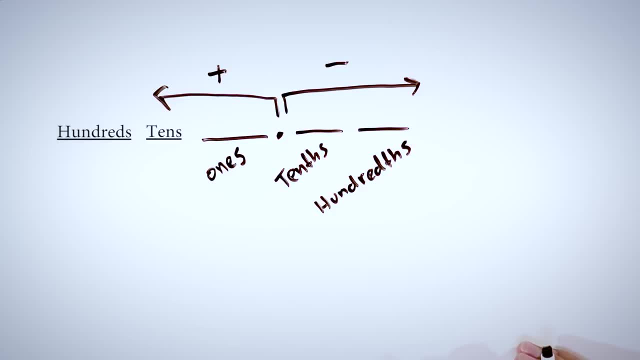 or our values will be decreasing. So let's go ahead and talk about the value of these places. All right, so let's go ahead and talk about the tens place first. So the tens place is right next to the ones place, separated by the decimal. So these are ones and. 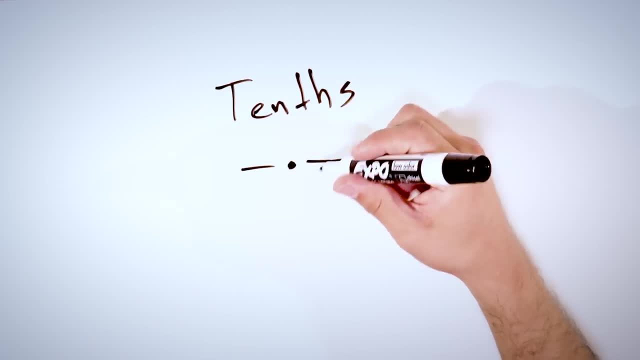 these are tenths, So we're going to talk about the value of just one tenth. I recommend putting a zero here to separate- um, not separate, but just to make the decimal a little more visible, because we don't have any whole numbers. so I just like putting the zero there just to make. 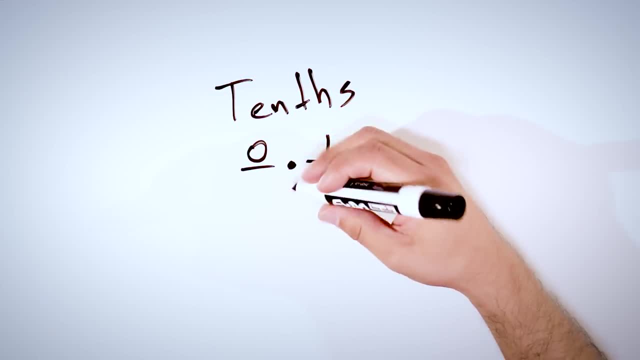 the decimal stand out more. So this is the tenths place here. so what is the value of the tenth place? Well, if you remember, we said that this is going to be less than the ones place. so what is actually smaller than a one? Well, we're going to have to. 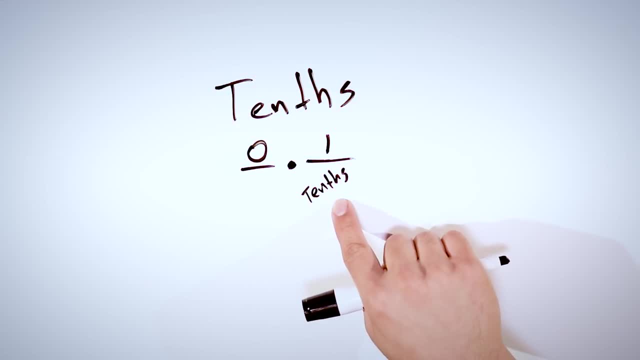 get into fractions. so the value of our tenths place is actually a fraction of one tenth, or one over ten. So that means that you need ten tenths to make a total of five tenths. So what one whole. And depending on your digit here, the fraction changes. So for example, you have two. 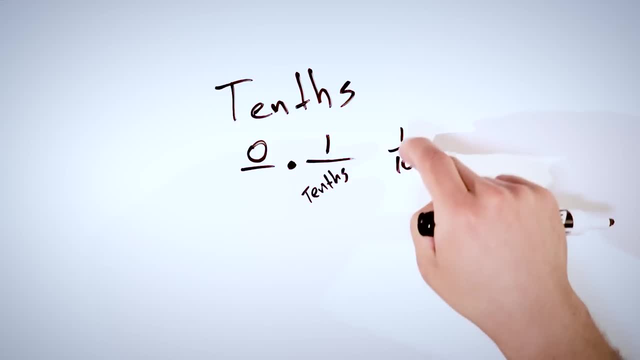 tenths, the fraction would be two tenths a three, three tenths, four, four tenths, five, five tenths and so on, And we will need ten tenths to make one whole. So the value of the tenths place is: 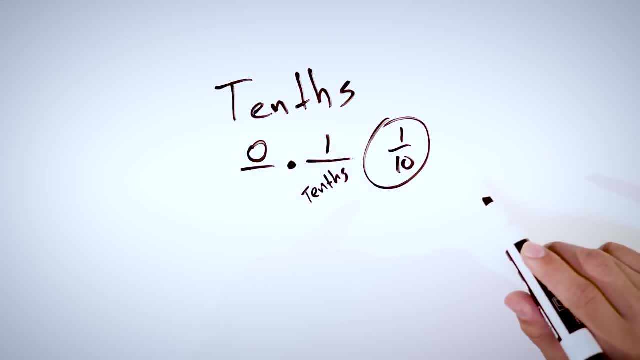 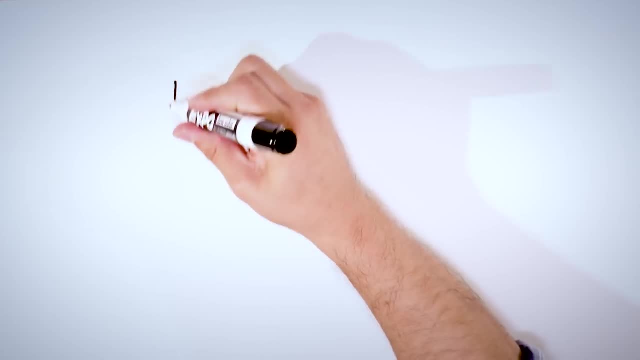 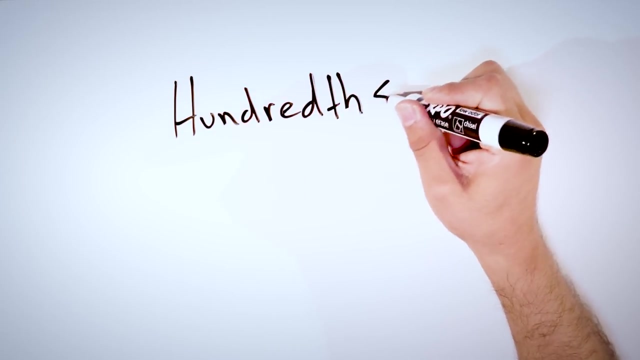 a fraction of one tenth. So let's go ahead and move on to the hundredths place. This one's a lot longer to spell, So give me a couple more seconds. Okay, sweet. So the hundredths place on the number on the number line, I'm sorry. on the place value chart.